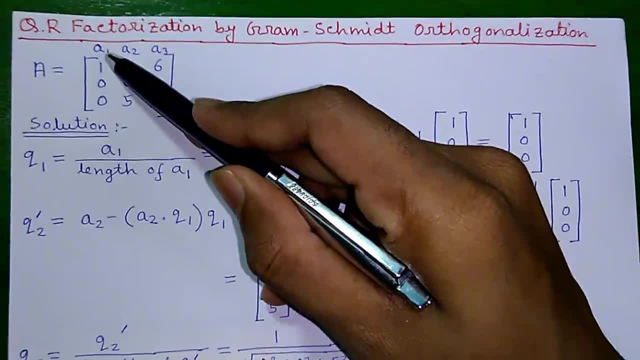 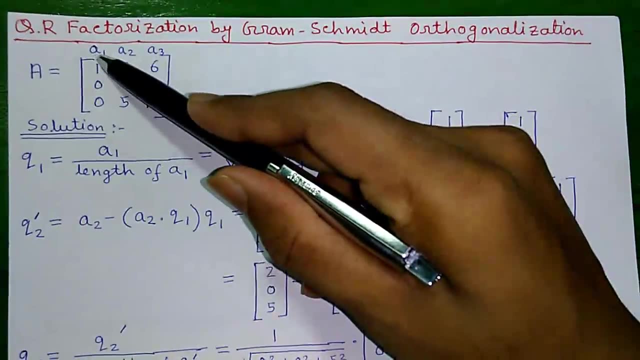 So first let me tell you column 1 of matrix A is called A1, column 2 called A2 and column 3 called A3. Here A1, A2, A3 represent the column vector. So let's proceed to the solution. 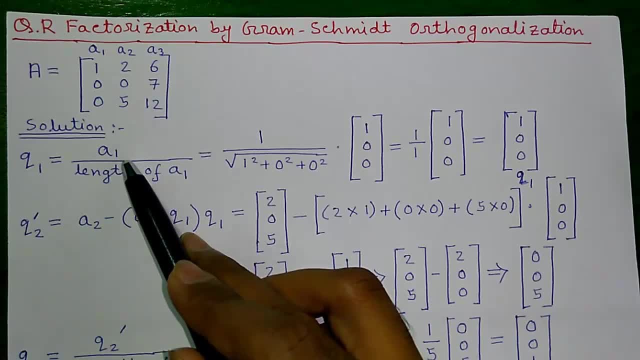 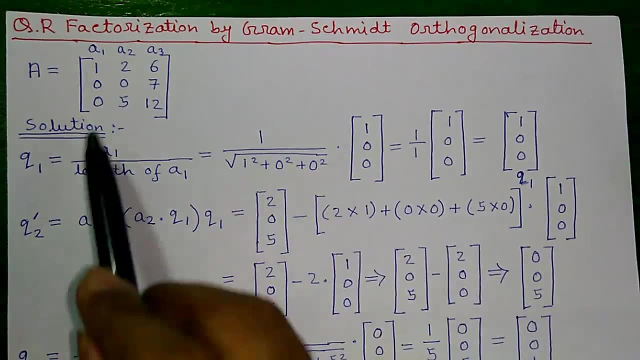 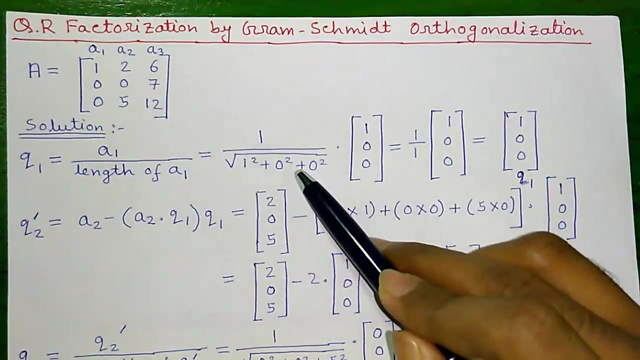 First we will calculate Q1, which is given by vector A1, divided by length of vector A1, which is equals to 1 divided by root over 1 square plus 0 square plus 0 square into A1, which is equals to 1 by 1 into A1, that is 1: 0.. 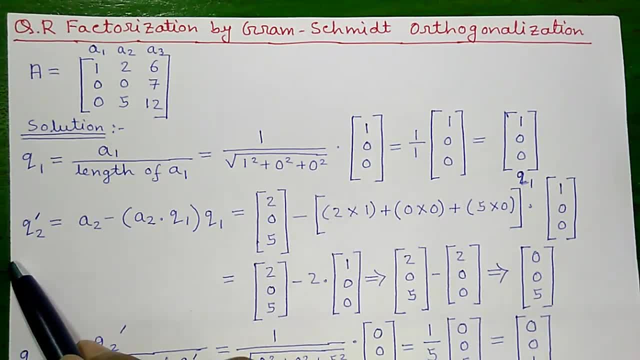 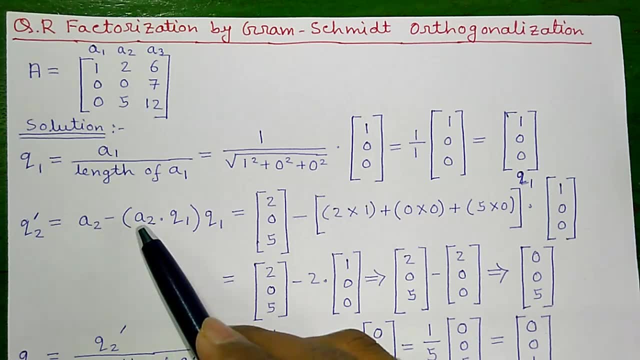 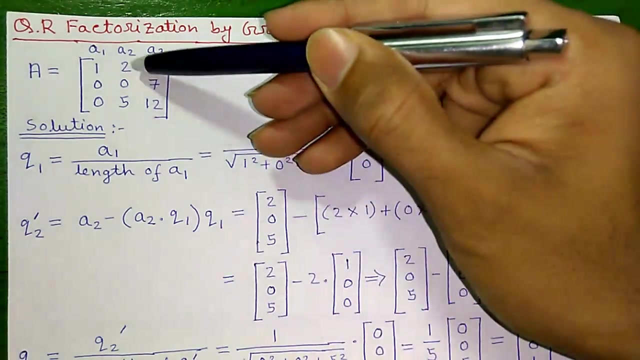 0, 0 is our Q1.. Next we will calculate Q2 in two steps. First we will calculate Q2 prime, which is equals to A2, minus A2 dot Q1 into Q1.. Here A2 dot Q1 represents the dot product of vector A2 and Q1, which is equals to A2- that is 2, 0, 5 is our second column- minus dot product of A2 into Q1. 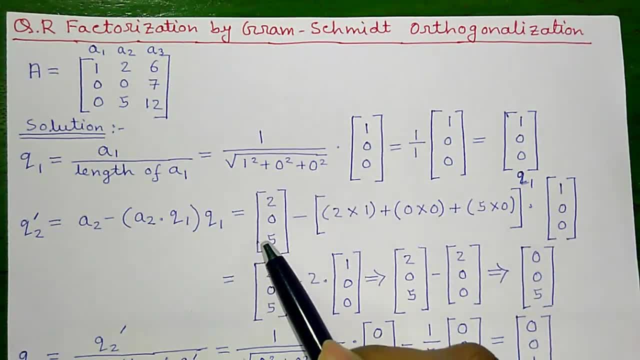 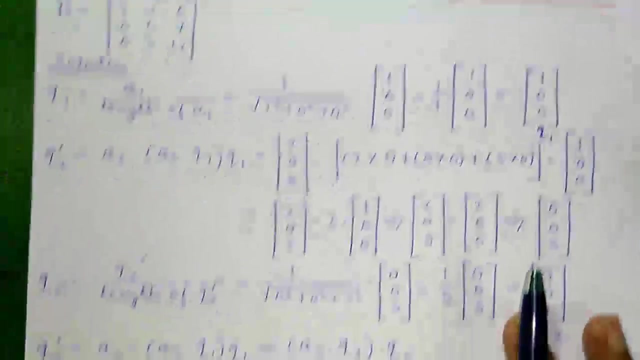 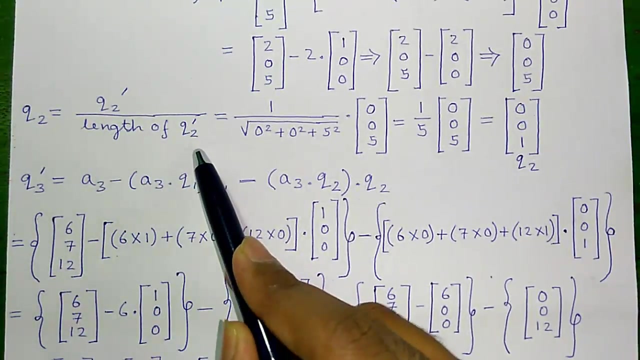 Here We will calculate Q1 costs. after this is equals to: 2 minus 2 is 0, 0 minus 0 is 0, and 5 minus 0 is 5. our quarry lecture is our q2 prime. Next we will calculate q2, which is equals to q2 prime divided by length of q2 prime. 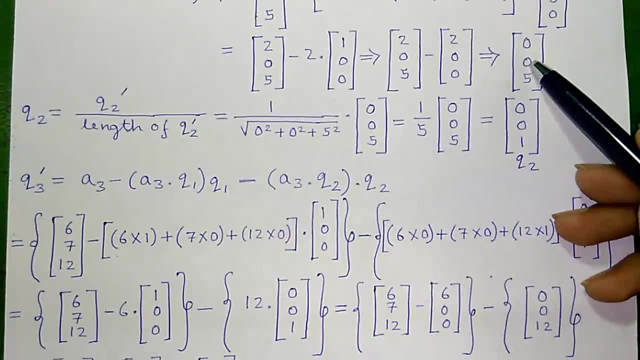 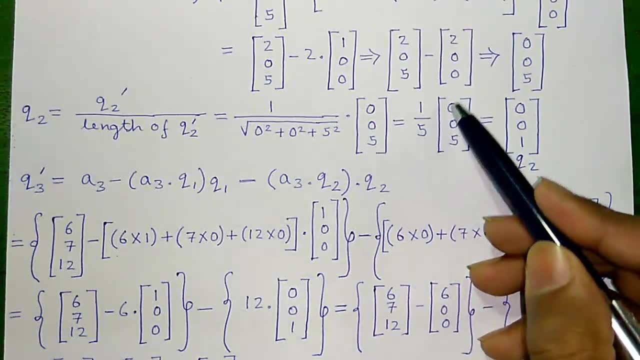 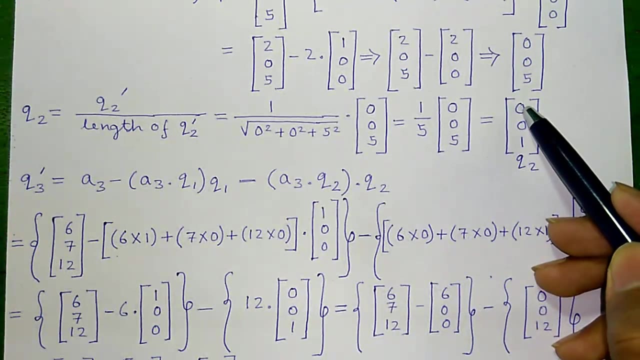 So that is equals to 1 divided by root over 0. square plus 0. square plus 5 square into q2 prime, that is 1 by 5 into q2 prime, that is 0 by 5, 0 by 5 and 5 by 5 equals to 0, 0 and 1 is our q2.. 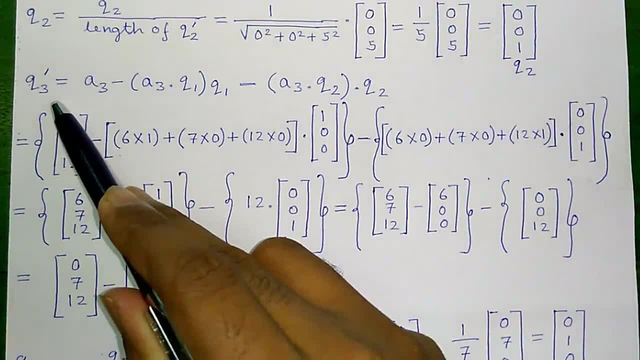 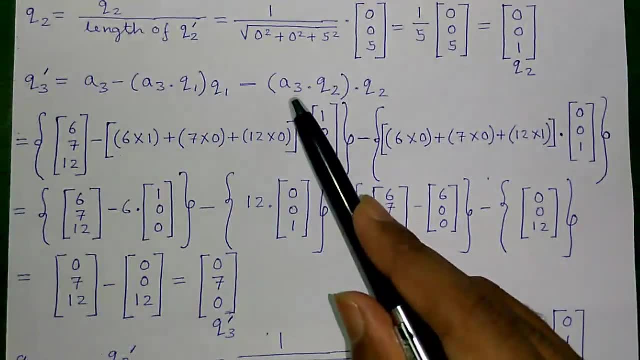 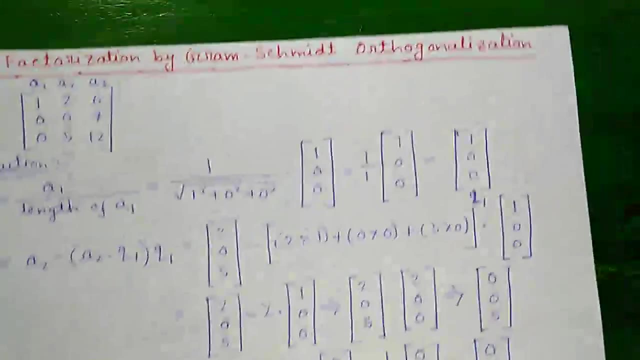 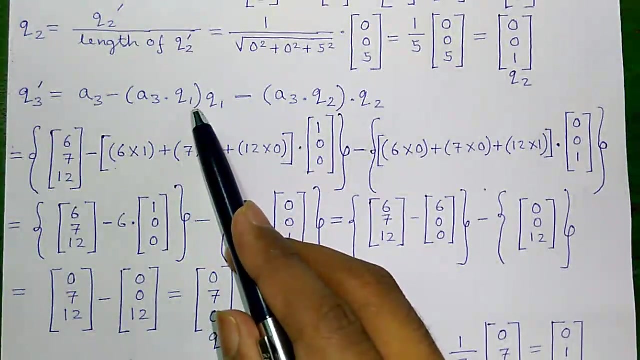 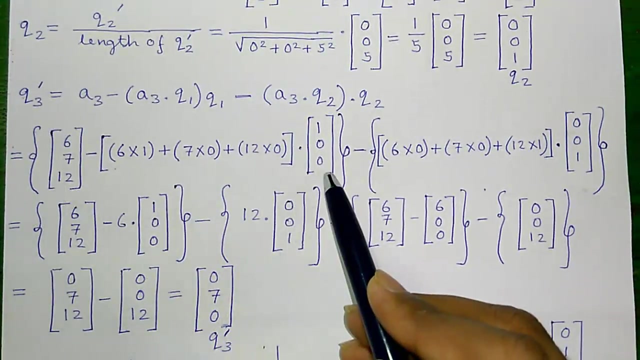 Similarly, we will calculate q3 in two steps. First we will calculate q3 prime, which is equals to h3 minus h3, dot q1 into q1, minus h3, dot q2 into q2.. So this is our h3.. Our third column, minus dot product of h3 and q1, that is 6 into 1 plus 7 into 0 plus 12 into 0. 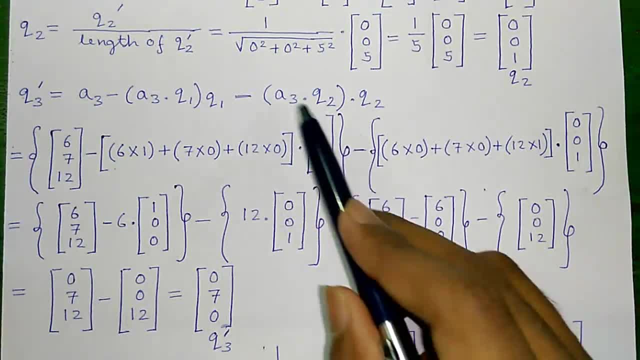 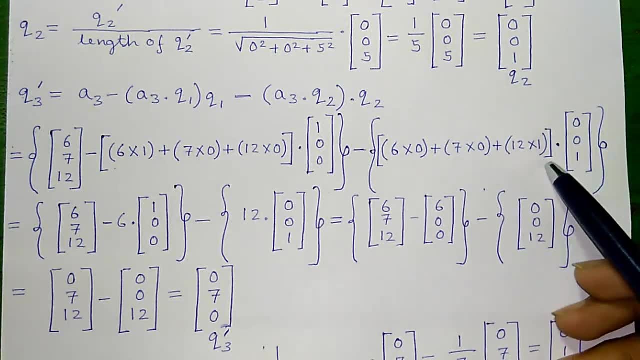 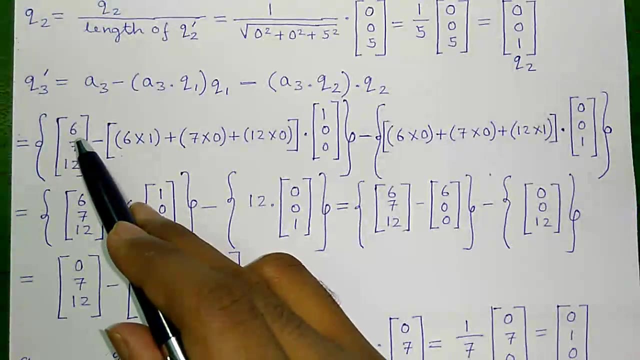 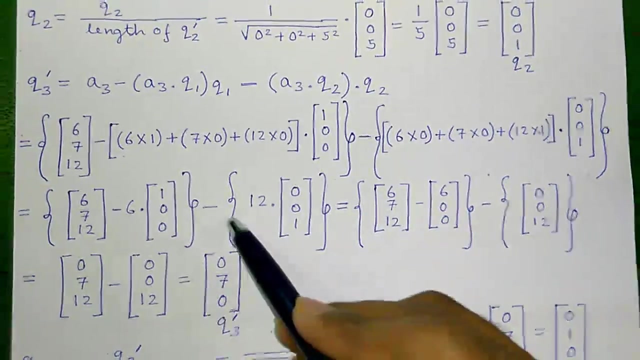 into q1 minus h3 dot q2, that is, 6 into 0 plus 7 into 0 plus 12 into 1 into q2.. So this equals to: So this equals to 6.. So h2, h3 minus 6 into q1. minus this equals to 12 into q2.. 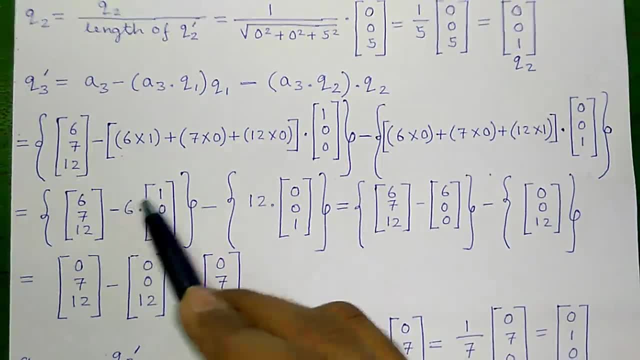 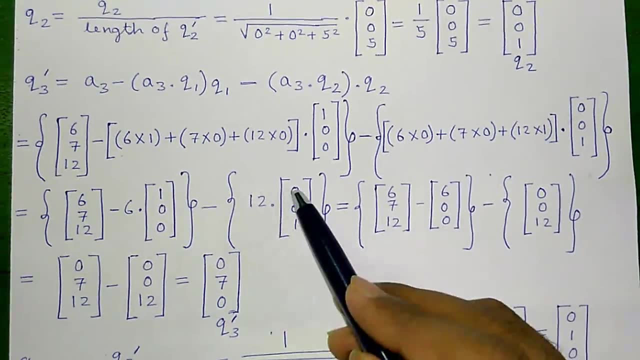 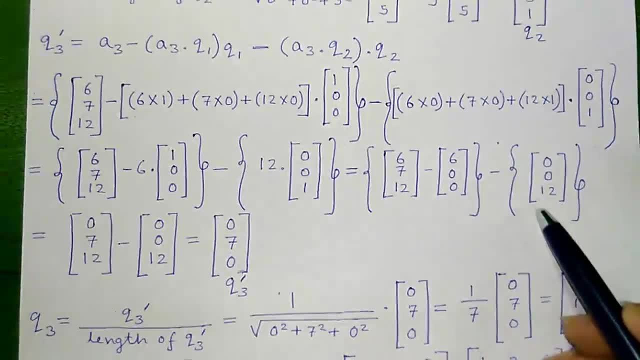 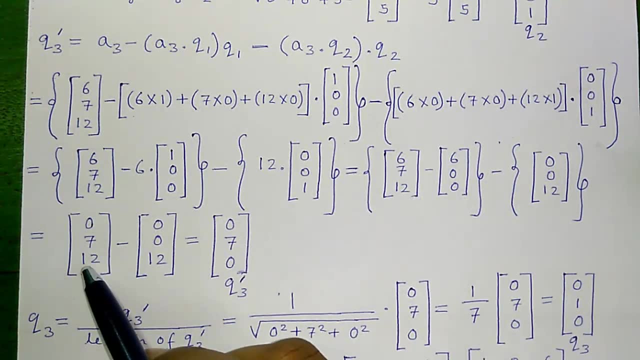 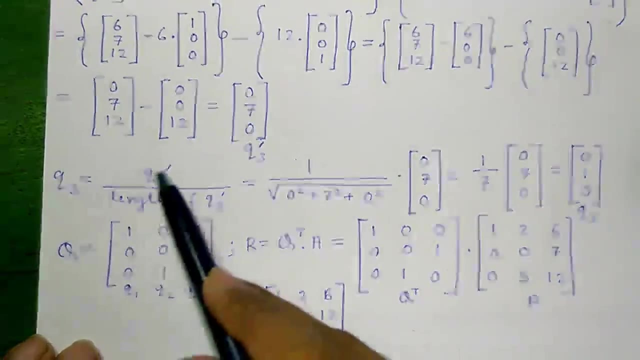 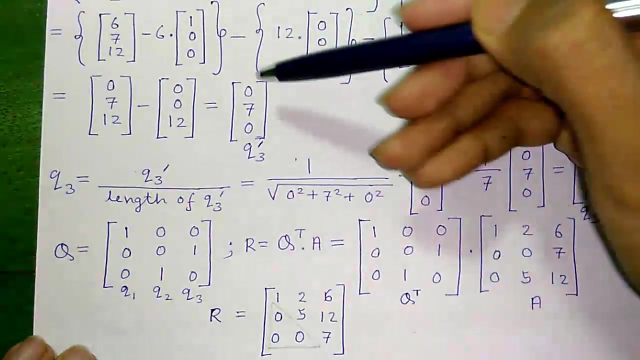 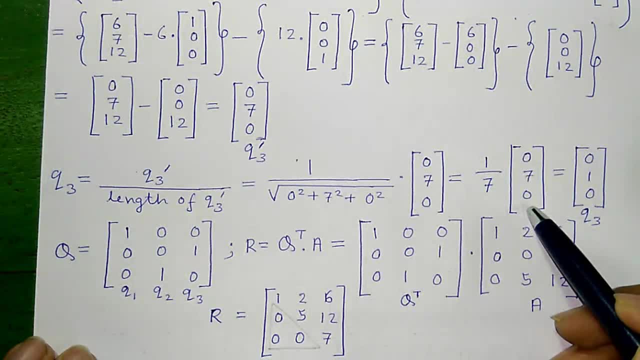 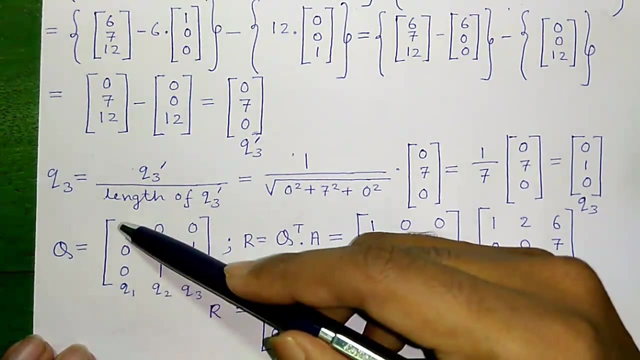 that is equal to 1 by 7, into Q3 prime, which is equal to 0 by 7, 7 by 7 and 0 by 7, that is 0,. 1, 0 is our Q3.. So we have got the sub-matrix Q, which is given by writing the Q1, Q2 and Q3 column wise. 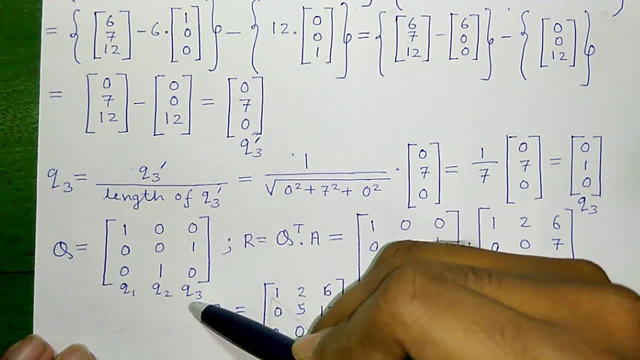 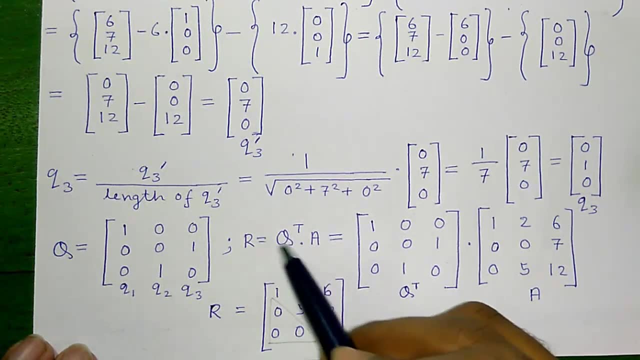 So column 1 is Q1, column 2 is Q2 and column 3 is Q3.. Next we will calculate sub-matrix R, which is given by Q transpose, into matrix A. Q transpose is given by row 1 of Q becomes column 1 of Qt 1, 0, 0, 1, 0, 0.. 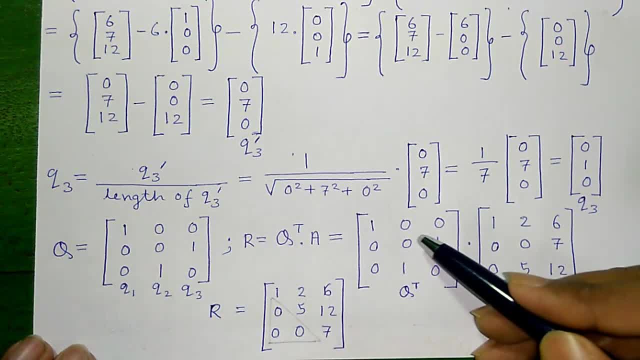 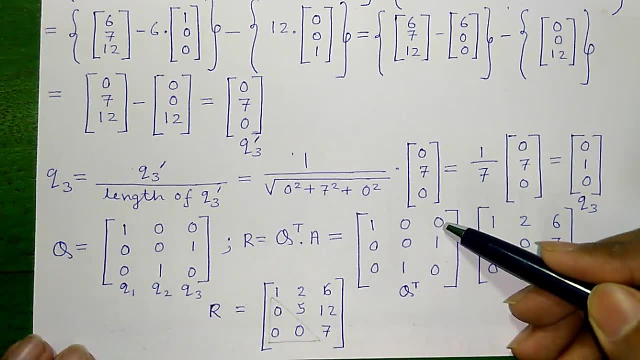 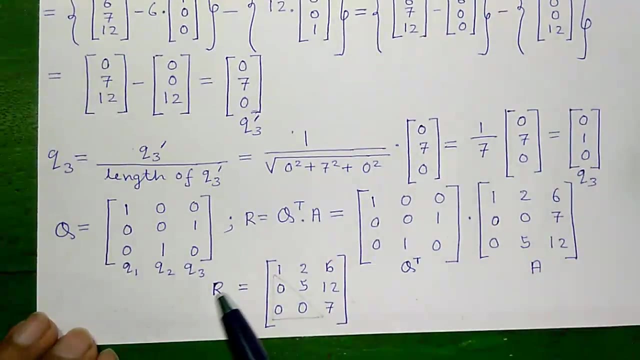 Row 2 of Q, that is 0, 0, 1, becomes column 2 of Qt: 0, 0, 1.. Row 3 of Q: 0, 1, 0.. So this is Q transpose into original matrix A, which is equal to sub-matrix R. 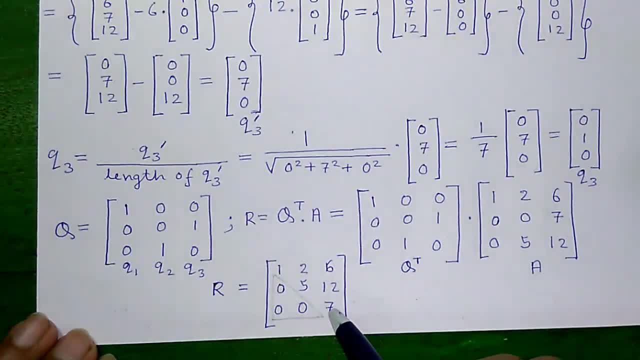 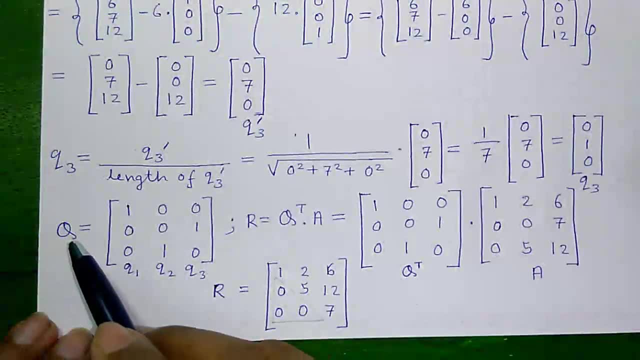 Here, matrix R is a upper triangular matrix. that means values are there in the upper triangle and lower triangular values are 0.. And Q is the orthogonal matrix and all the columns of Q are the orthogonal. That means they are linearly independent of each other. 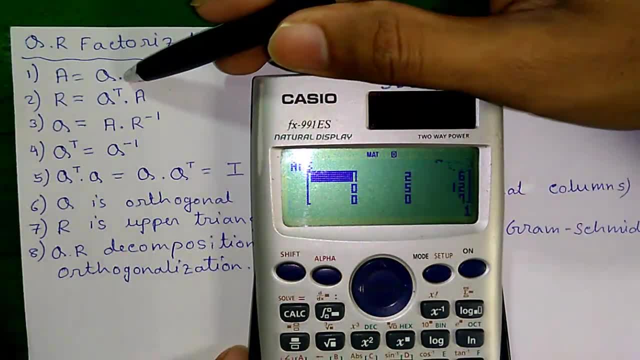 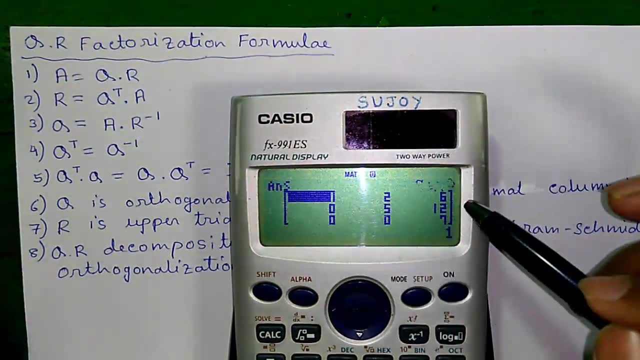 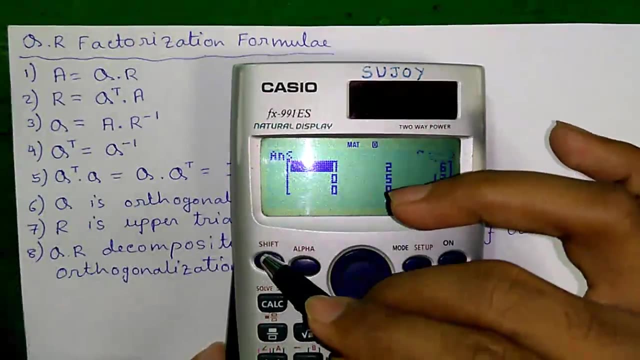 Now some properties of QR factorization. Property number 1, matrix A is equal to matrix Q into matrix R. So this is our matrix R which is stored as matrix. answer: You can directly store this matrix as matrix C on this calculator. For that, press shift rcl and enter the matrix name you want to save it to. 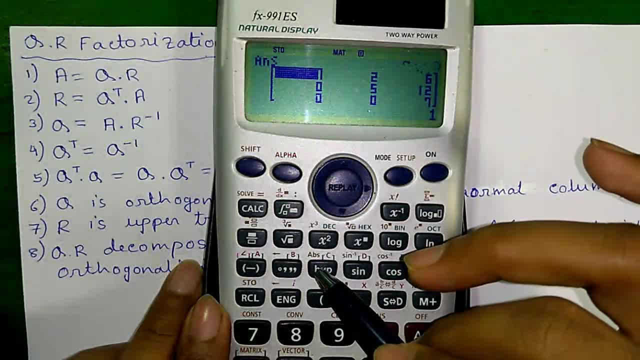 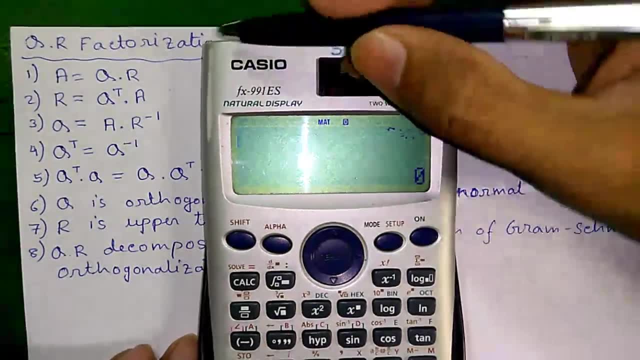 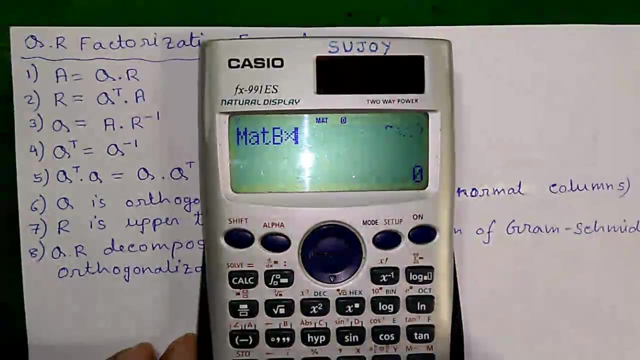 So this button for matrix A, this button for matrix B and this button for matrix C, Press this button So you can see it changed to C. So A equals to Q into R, Q is matrix B into C, is matrix R. Press equals to. 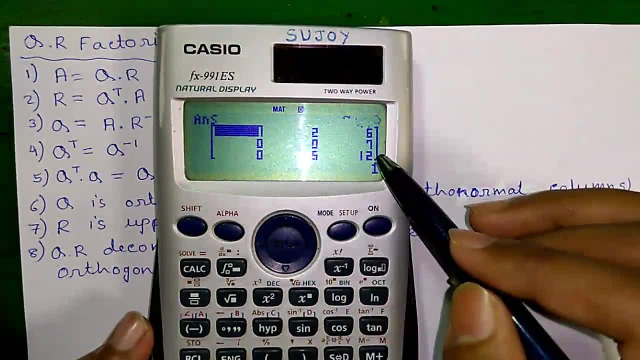 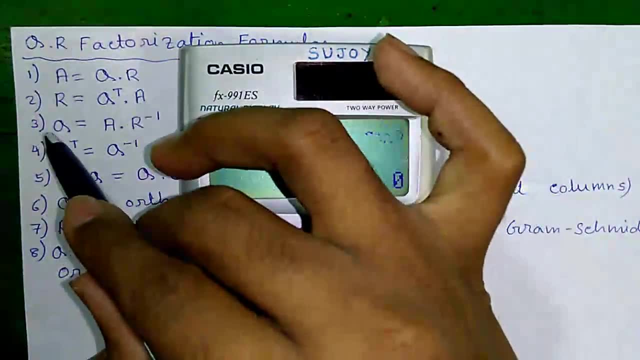 We have got our matrix A back: 1,, 2,, 6,, 0,, 0,, 7,, 0,, 5,, 12.. This button is matrix B, Press 2.. This property we use to find out the matrix R. 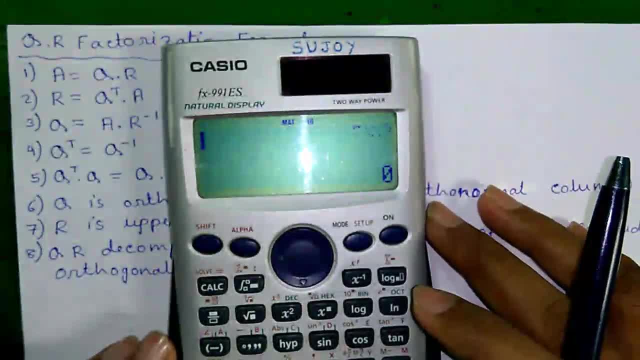 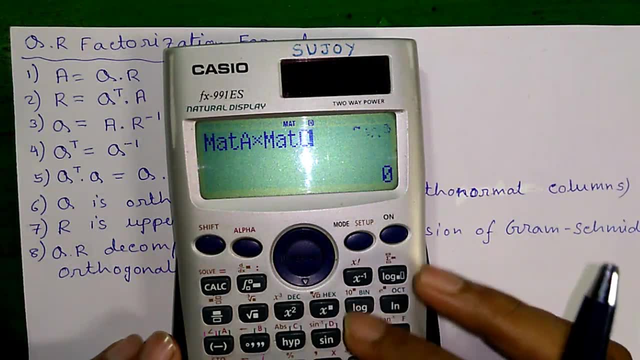 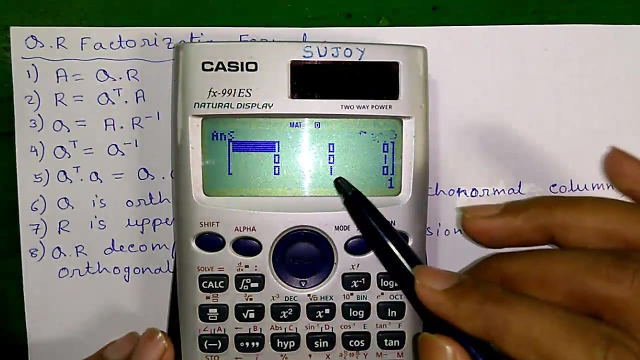 3rd property: Q equals to A into R inverse. So matrix A into R is matrix C inverse. That equals to Q 1, 0, 0, 0, 0, 1 and 0, 1, 0.. 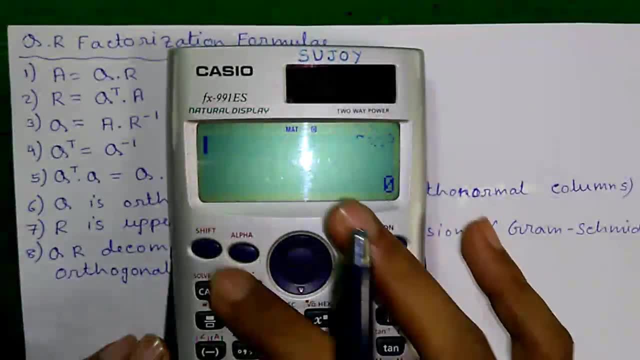 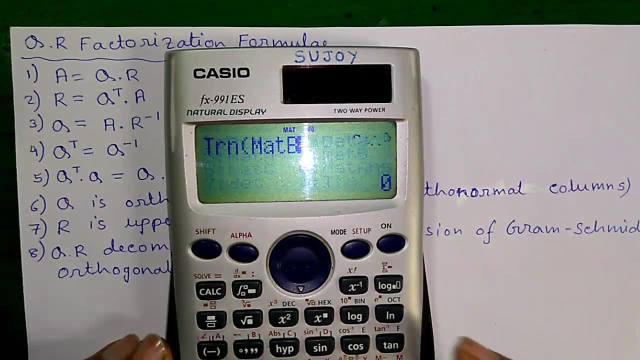 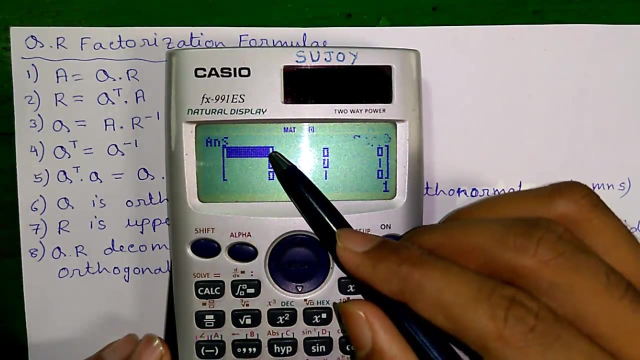 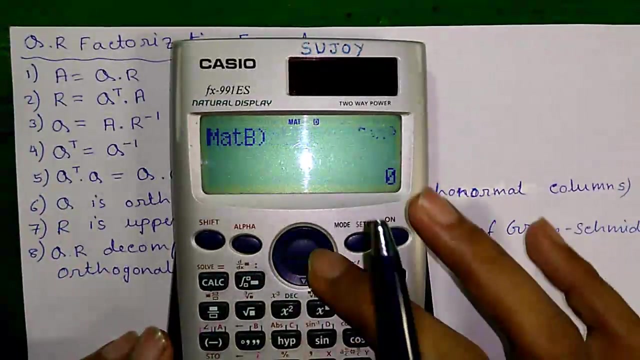 4th property: Q transpose equals to Q inverse 8 for transpose. So Q transpose is 1, 0, 0, 0, 0, 1 and 0, 1, 0.. Let's find out Q inverse. 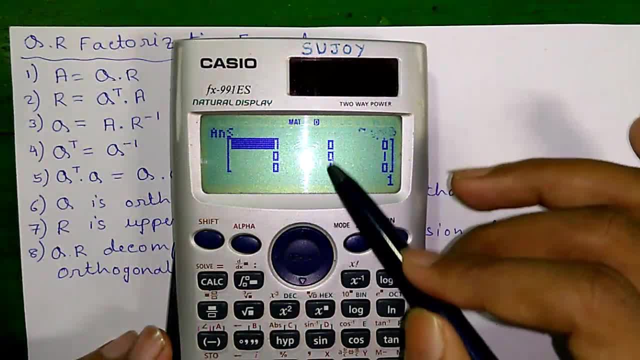 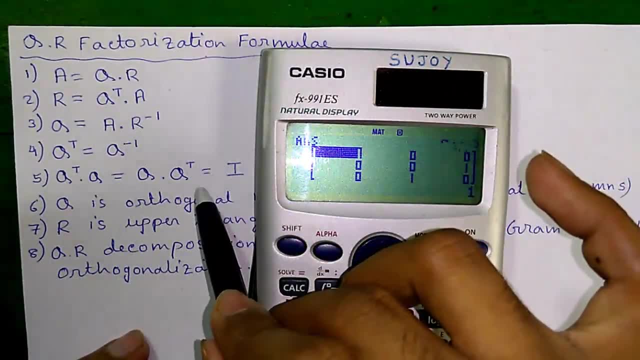 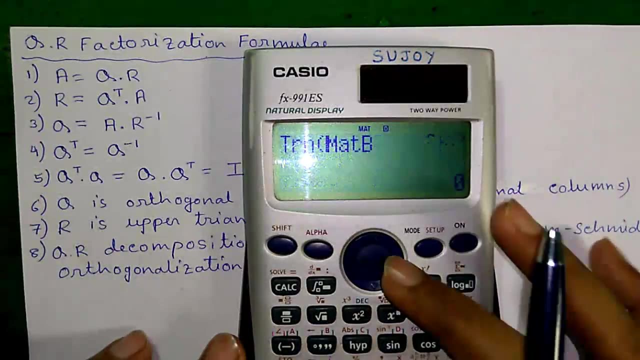 Press equals to, That is 1, 0, 0, 0, 0, 1 and 0, 1, 0.. 5th property: Q. transpose into Q equals to Q into Q. transpose equals to matrix R.